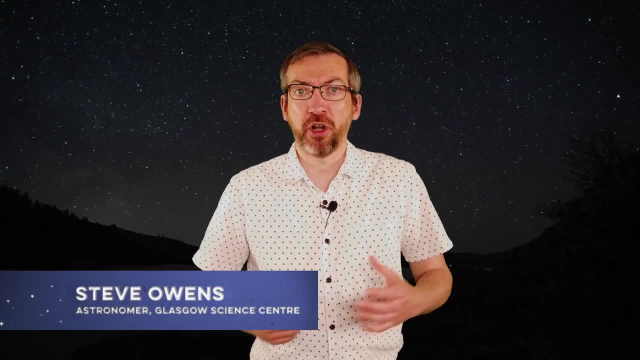 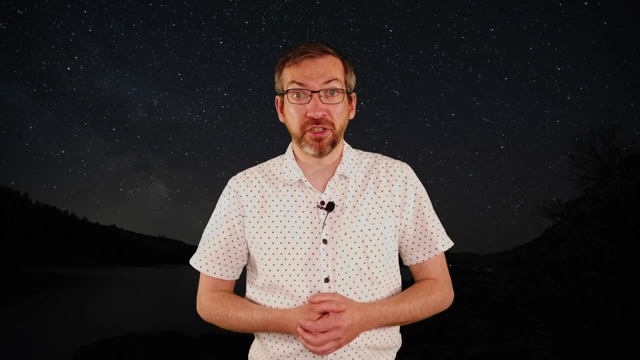 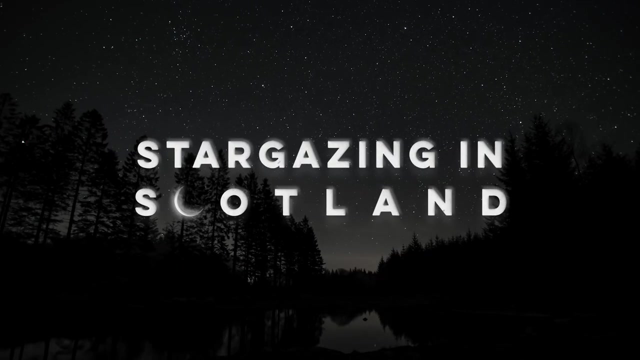 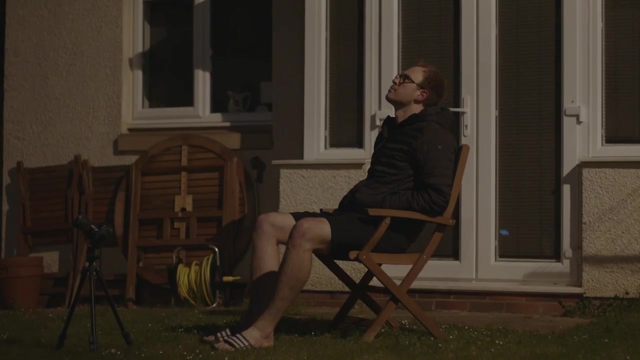 Hello, my name's Steve. I'm an astronomer at Glasgow Science Centre and welcome to Stargazing in Scotland, introducing you to the night sky from a Scottish perspective. In this video, I'm going to focus in on six well-known and easy to identify constellations, so you can go and find them for yourself. 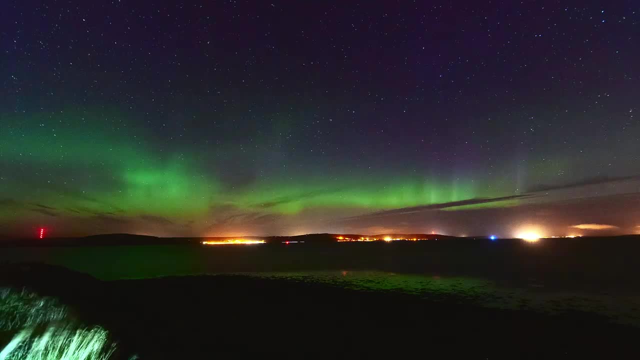 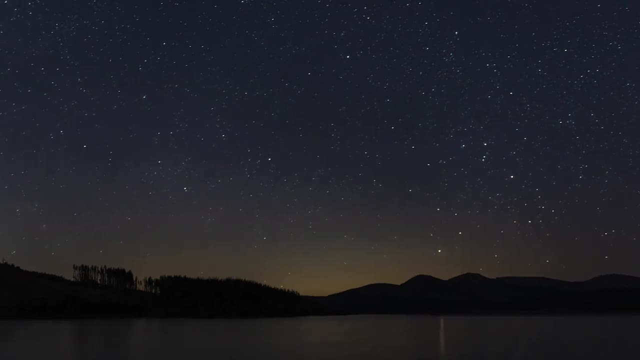 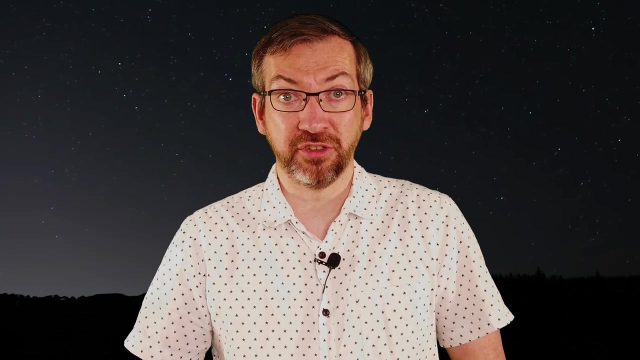 The sky changes over the course of a night. As the earth spins, the stars appear to rise and set. Over the course of a year. as the earth orbits the sun, different stars and constellations become visible in different seasons. There are 88 constellations altogether and from Scotland, some of those are seasonal. 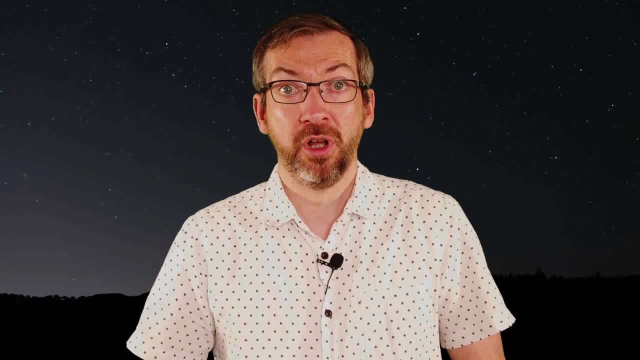 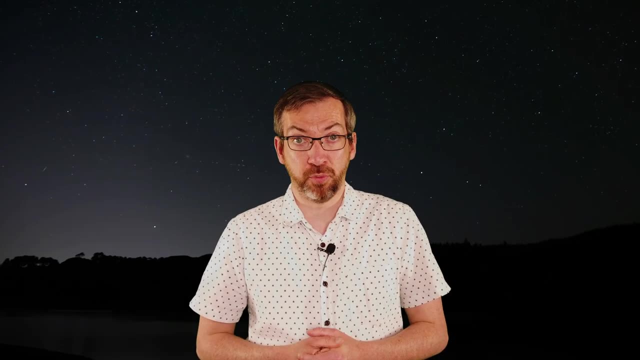 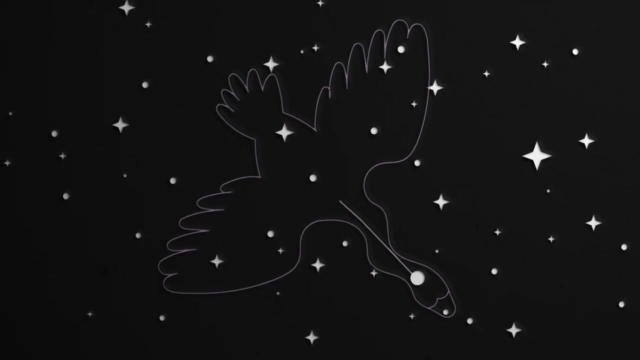 only seen in specific months of the year, whereas others are visible all year round. Let's begin in the summer in Scotland with one of the easiest to find summer constellations: Cygnus the Swan. Cygnus the Swan actually looks like its name suggests. It has a long neck that follows the 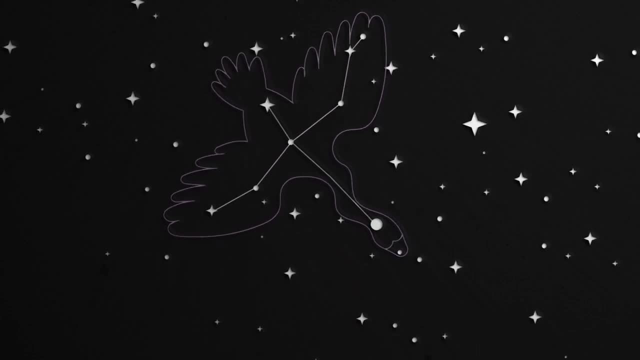 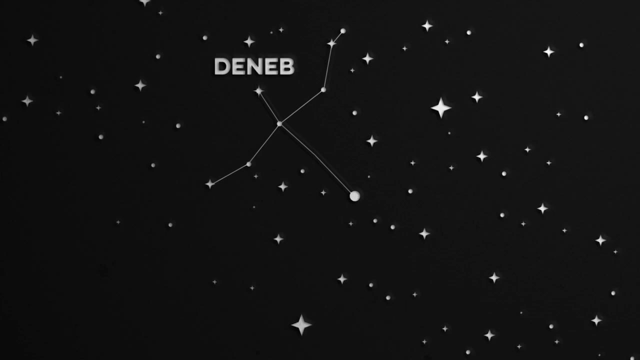 path of the Milky Way. two wings, one on either side and a tail behind. In the tail of the swan we find the star Deneb, the brightest star in Cygnus. Deneb is actually one of three stars that make up a pattern known as the Summer Triangle, best seen in Scotland in the summer. 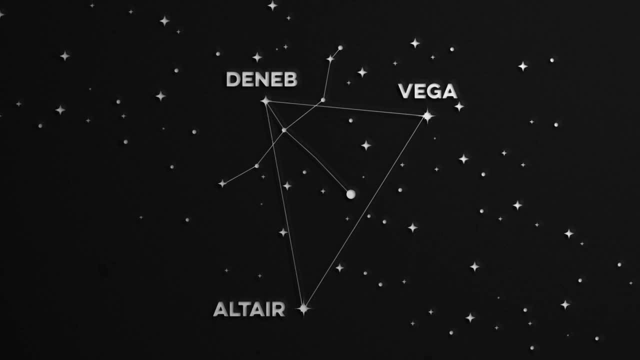 months. The three stars of the Summer Triangle are actually the three different constellations, So this isn't a constellation on its own. we call this pattern an asterism, Moving from summer to autumn. we're going to look at the constellation Pegasus, the wind horse. 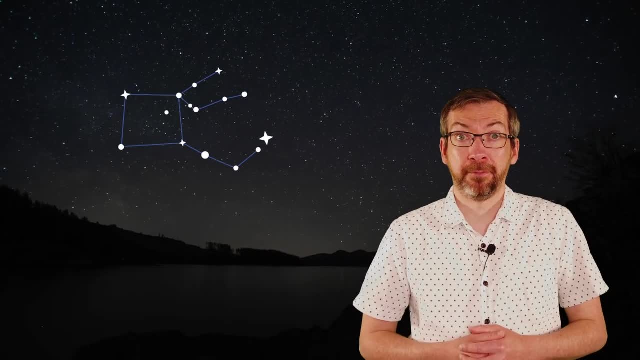 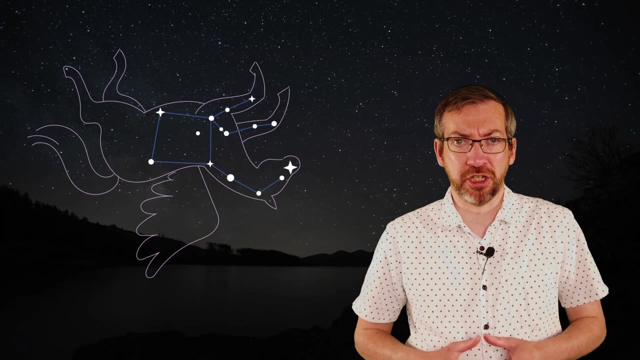 Pegasus also has a shape in it, this time a square. Now, if you struggle to see a swan when looking at Cygnus, you'll really struggle to see a wind horse when looking at Pegasus. I can usually only just see the four stars of the square, And coming out of the corner of that square is the constellation of Andromeda, the Princess. 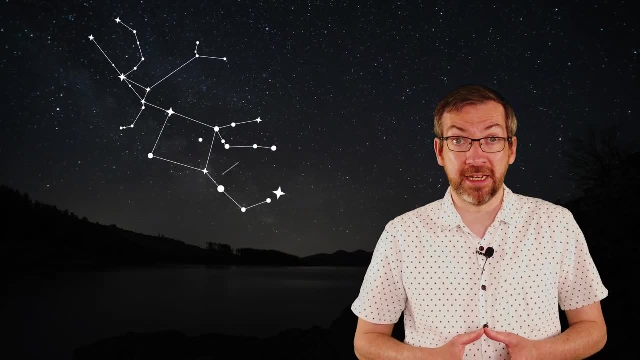 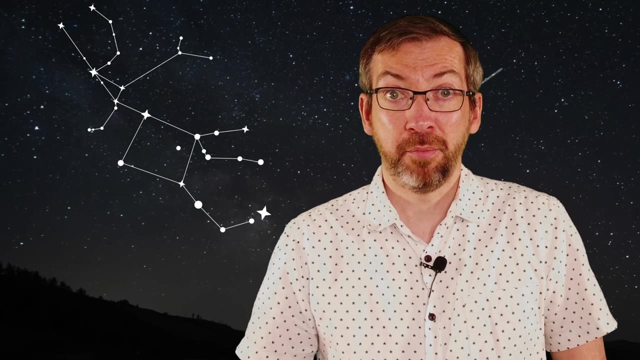 Andromeda the Princess is the constellation of Andromeda the Princess and the constellation of Andromeda the Princess, Home to the furthest thing you can see with the naked eye: the Andromeda Galaxy. The Andromeda Galaxy is actually quite hard to track down on its own because it is very faint. 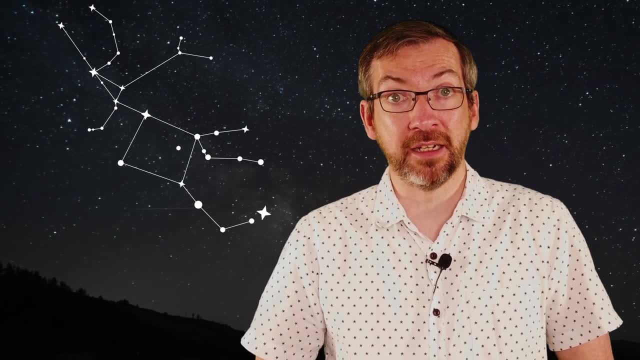 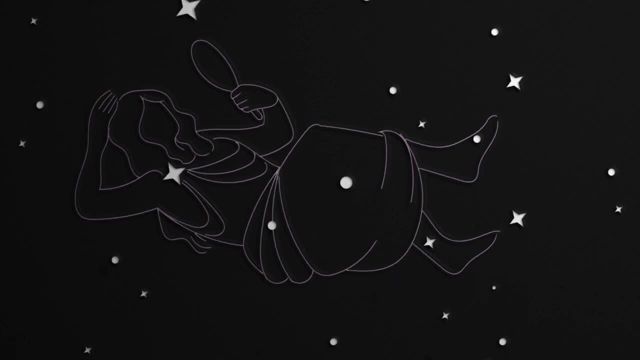 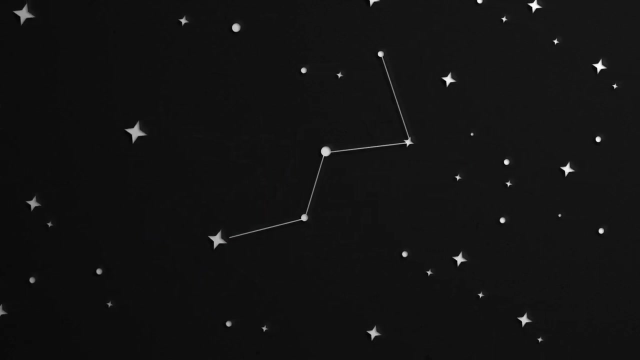 but you can use another constellation as a signpost to help you find it. That is Cassiopeia. In Greek myth, Cassiopeia, the Queen, was the mother of Andromeda. The constellation Cassiopeia is made up of five bright stars in a distinct W shape. The right-hand V of that W acts as a. 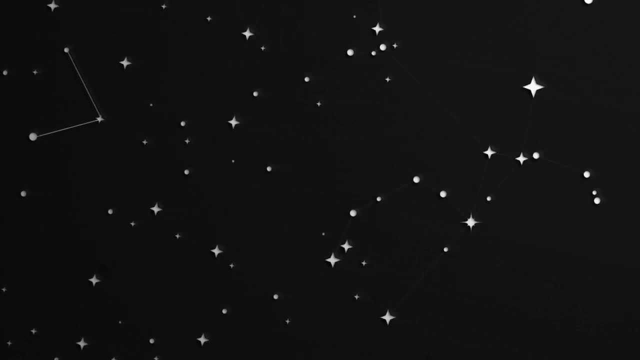 symbol and the left-hand V acts as an arrow that points us to the middle three stars in the constellation of Andromeda. From that middle star hop one faint star up and the same distance again and you find the faint smudge of the Andromeda Galaxy, A collection of a trillion stars, that is, two and a half million. 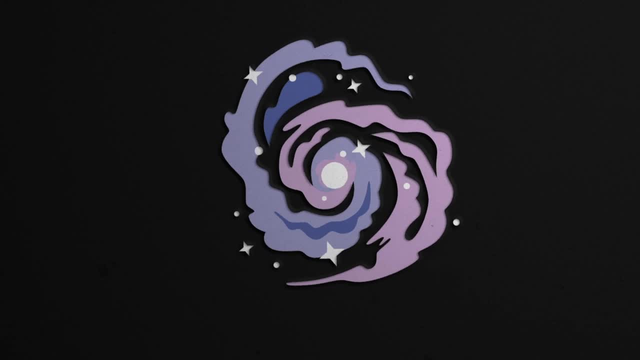 light-years from us And it's actually on a collision course. It's hurtling towards our galaxy, the Milky Way, But don't panic, it's not going to hit us for another few billion years, Moving from autumn into winter. Cassiopeia is a signpost for the Andromeda Galaxy. Cassiopeia is the first star in the Andromeda Galaxy, which is the biggest star in the Andromeda Galaxy. It's the second star in the Andromeda Galaxy. It's the third star in the Andromeda Galaxy. 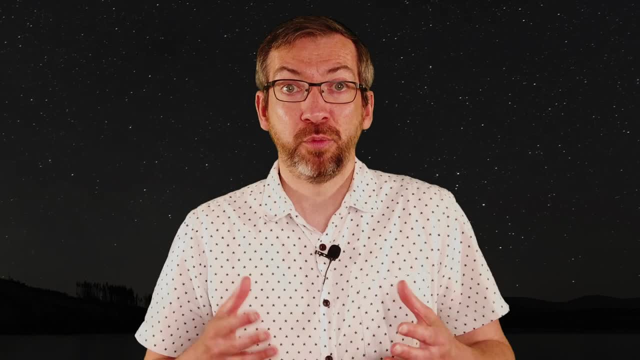 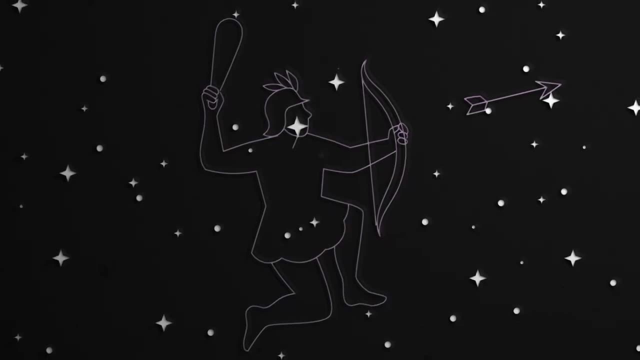 Moving from autumn into winter, we find one of the most spectacular constellations visible in Scotland, Orion, the Hunter. Orion has three stars and a belt: two stars for its shoulders, two for its feet. He has a curve of stars for a shield and a sweep of stars above his. 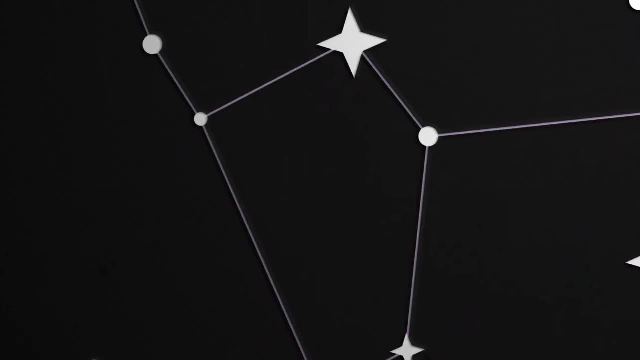 head as a club. The left-hand star of its shoulders is a star called Betelgeuse. It's got a very distinct orange-red colour, and that's because Betelgeuse is a dying star. It's running out of hydrogen fuel and as it does so, it's expanding, cooling down and 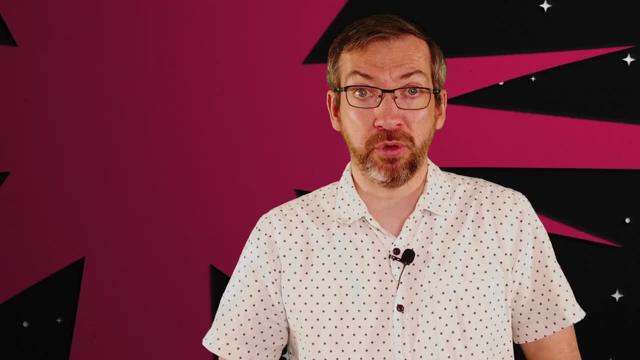 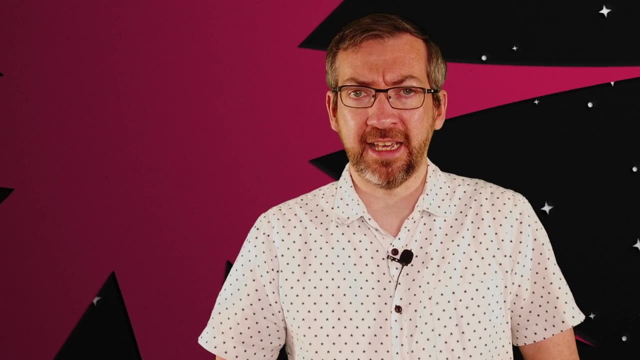 turning red. Any day now Betelgeuse will explode in what we call a supernova explosion, lighting up the sky. Now you should be suspicious astronomers when we say any day now, For us that's some time in the next million years. Probably won't happen tonight, probably won't. 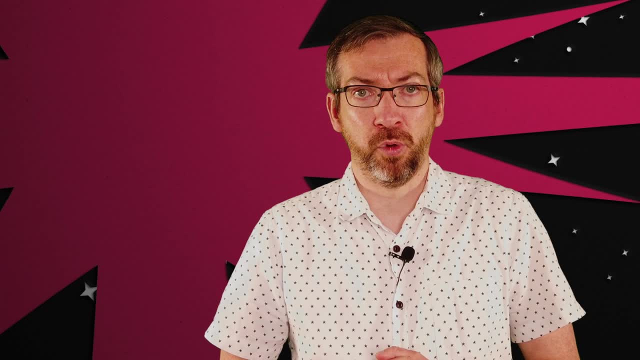